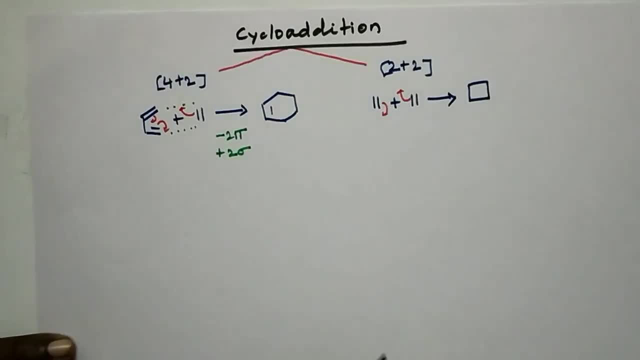 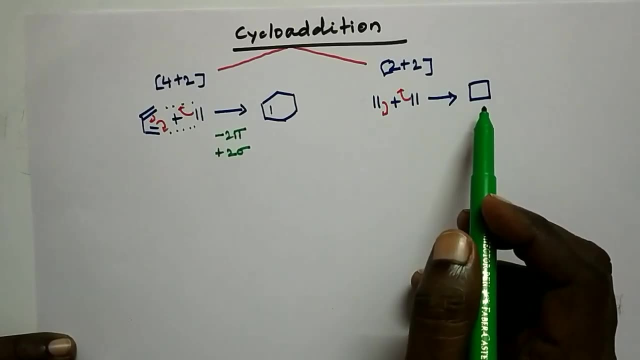 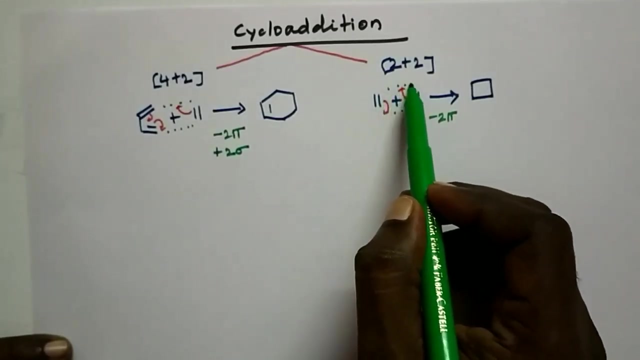 means two sigma bonds are gained. And look at this: one: 2 plus 2.. How many pi bonds? Two And here 0. That means we lost 2 pi bonds. Sigma bond: here one sigma bond, here another sigma bond. 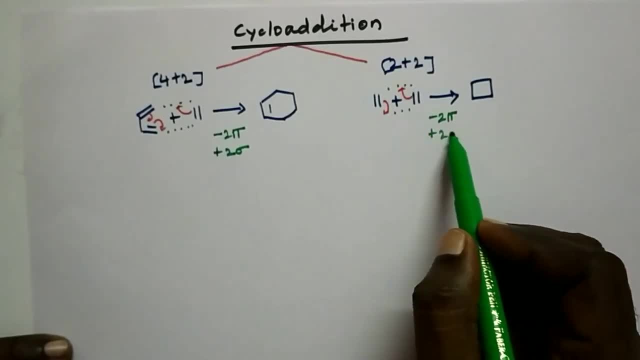 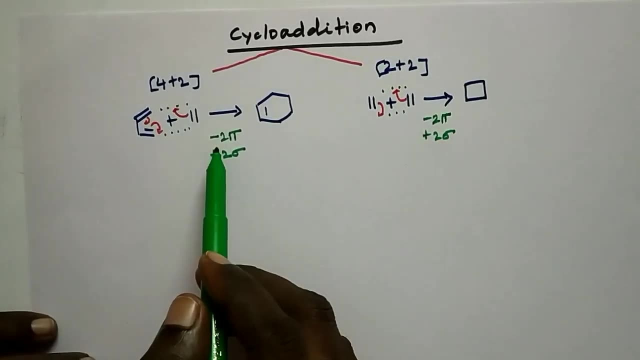 are newly forming. So gain of 2 sigma bonds. Okay, So basically, in both the cases you see. similarly, we lost 2 pi bonds in both the cases. We gained 2 sigma bonds in both the cases. So this is a. 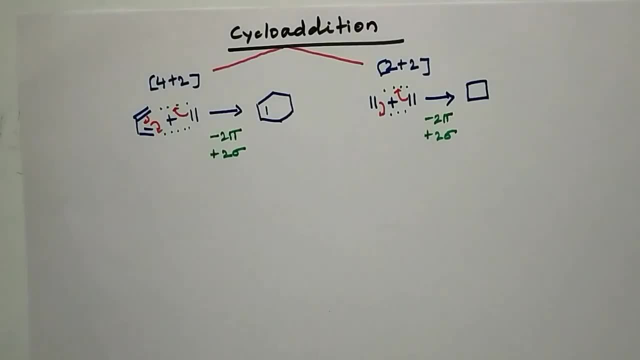 typical attribute of cycloaddition reactions. Okay, Now we are going to see how the orbitals involve in the cycloaddition reaction, Because we have been right. from the first video we have been seeing the involvement of orbitals homo lumo symmetric. 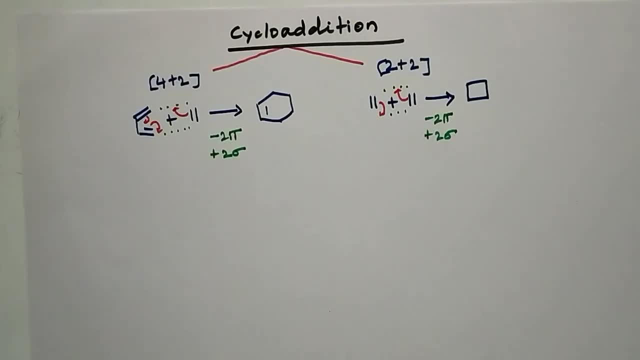 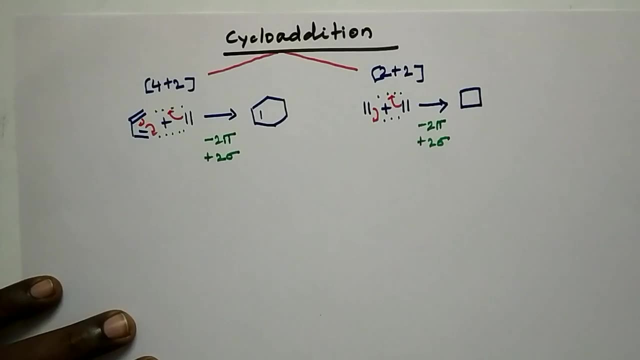 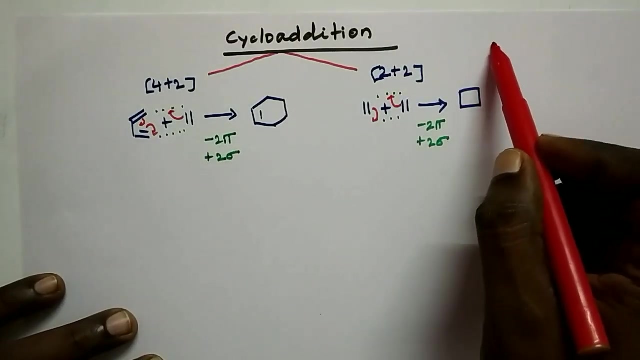 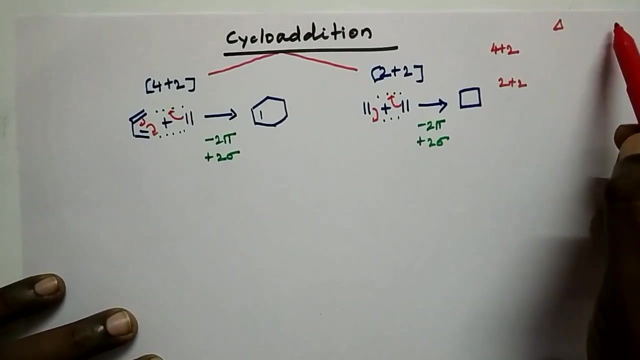 asymmetric, plenty of things. How are we going to apply all those things? And according to Woodward-Hoffman rule- remember Woodward-Hoffman rule- 4 plus 2 and 2 plus 2, thermally, photochemically, Okay. 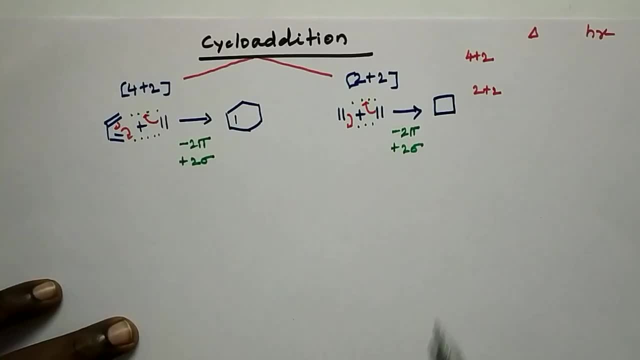 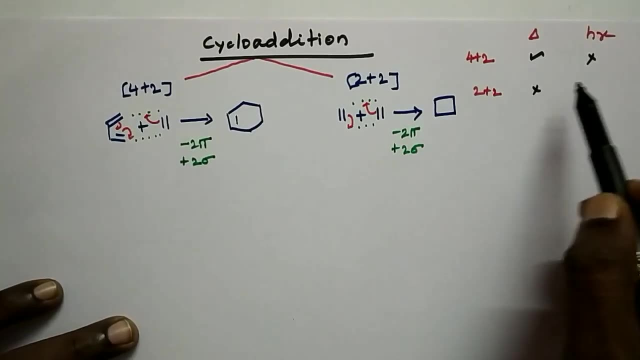 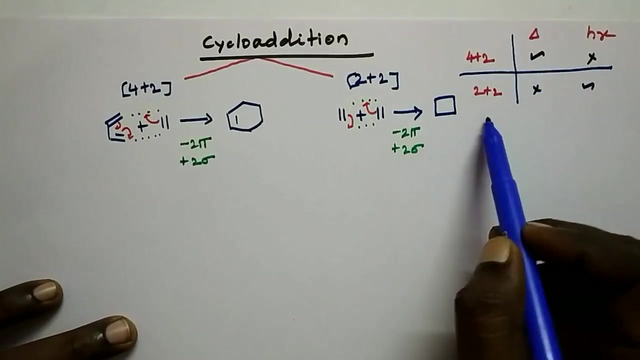 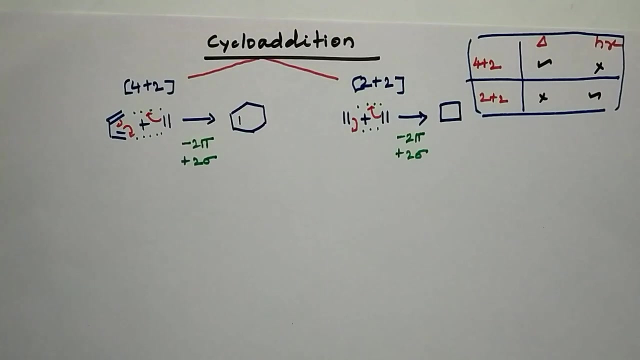 4 plus 2: reaction is thermally allowed. photochemically forbidden. 2 plus 2: cycloaddition is thermally forbidden. photochemically allowed. Okay, You need to remember this rule. 4 plus 2- thermally allowed. 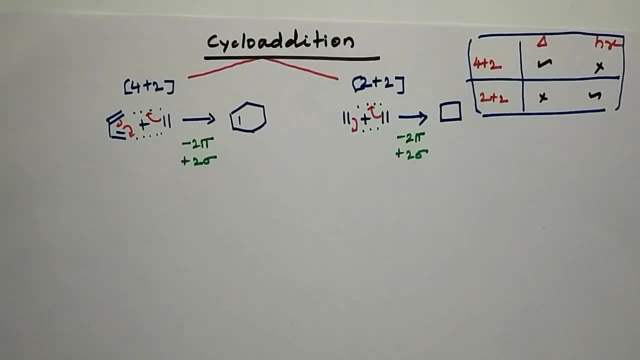 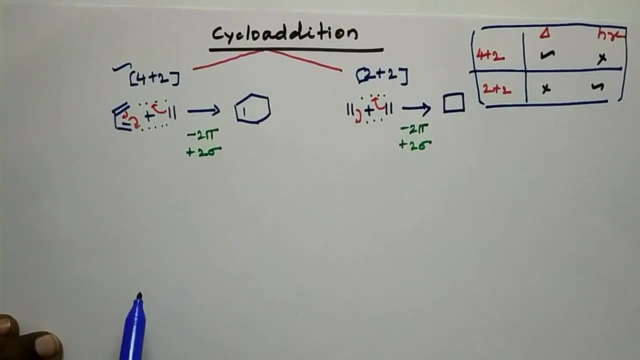 2 plus 2 photochemically allowed. How is it? came to know? came to be: Okay, Let's see. First of all, let us deal with 4 plus 2 cycloaddition. Okay, Let us take this one. 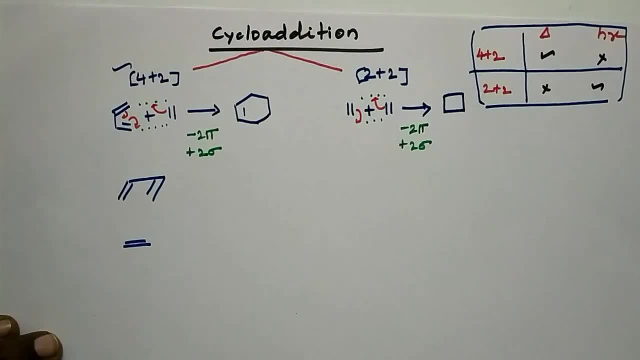 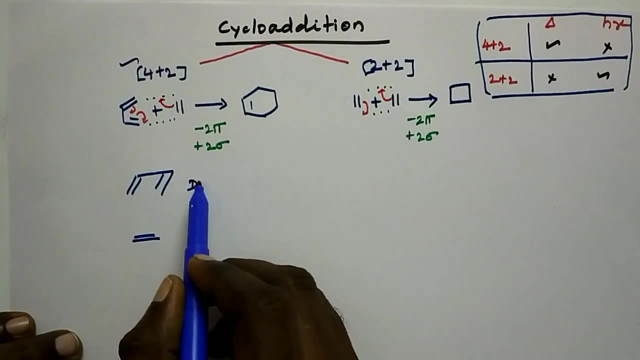 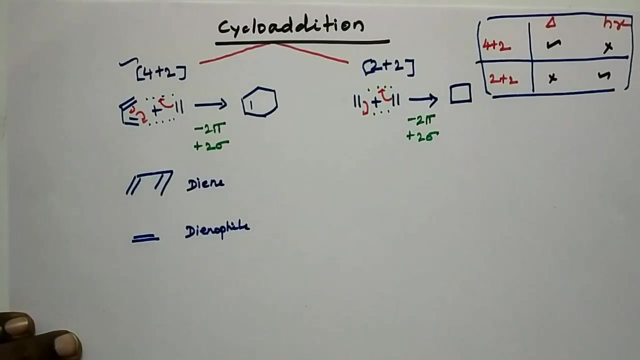 And okay, this one is called diene. Okay, This one is called diene. The other one is called dienophile. Dienophile- Okay, Dien dienophile- Okay, They both add thermally: What will happen? 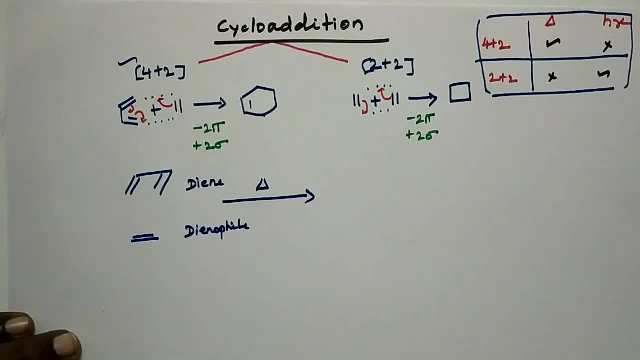 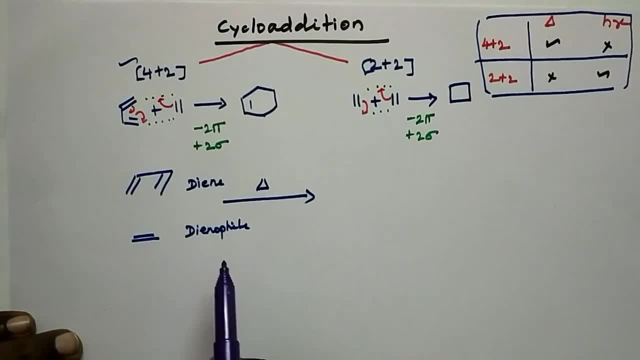 look at the orbitals. As I said, if it is thermal condition, you need to take homo and lumo. Okay, Homo is the highest occupied orbital, Lumo is lowest unoccupied orbital. So so that from homo to lumo, 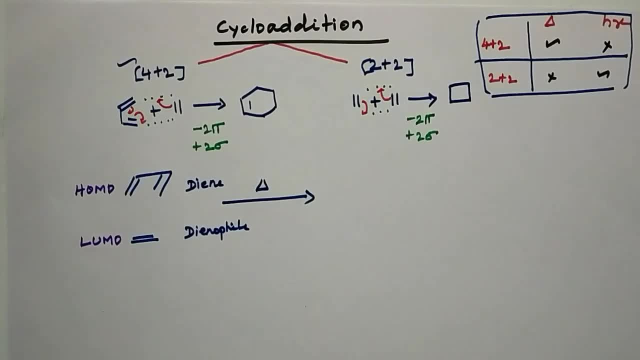 electron can be transferred, to generate, to make bonds. Okay, So that is why homo and lumo involve. We take lumo of dienophile, homo of diene, Okay, How can it draw HOMO? and how can we draw the LUMO? Remember, everyone loves Neha, old heroine. 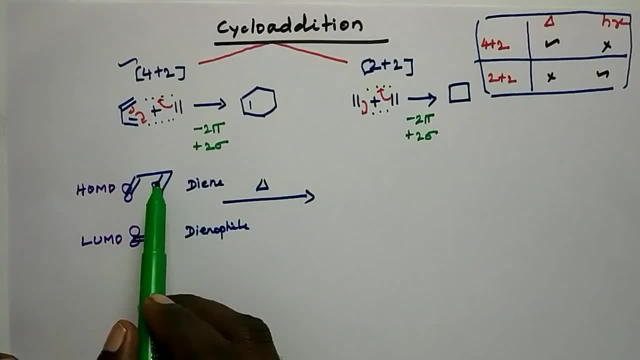 Sridevi, I hope you remember that. okay, Two pi bonds, that means even number E1. LUMO symmetric, LUMO symmetric means HOMO asymmetric. and come here, Here: LUMO is asymmetric, LUMO is asymmetric, HOMO asymmetric, LUMO asymmetric. So if that 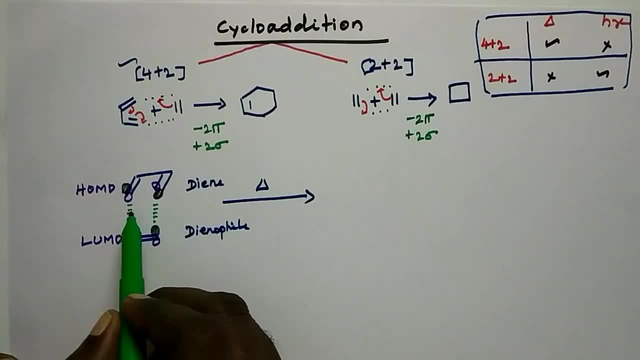 is the case. there is orbital, okay, symmetry matching. So this is supra, Supra, Supra facial. okay, Supra facial. is symmetry allowed, Always remember, especially for 4 plus 2 and these two cycloadditions, 4 plus 2 and 2 plus 2.. 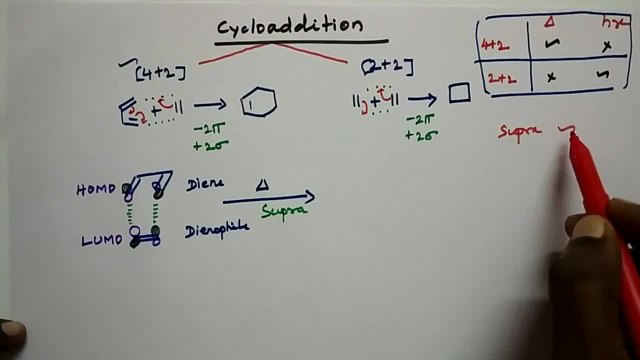 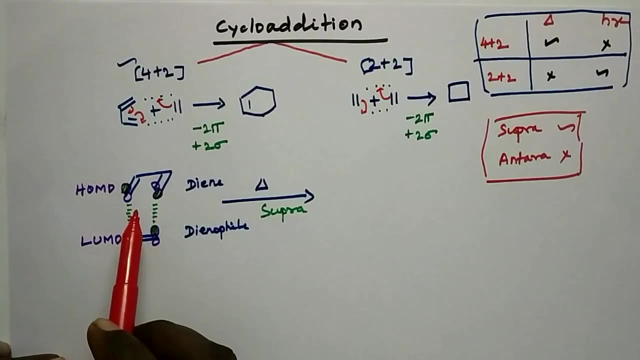 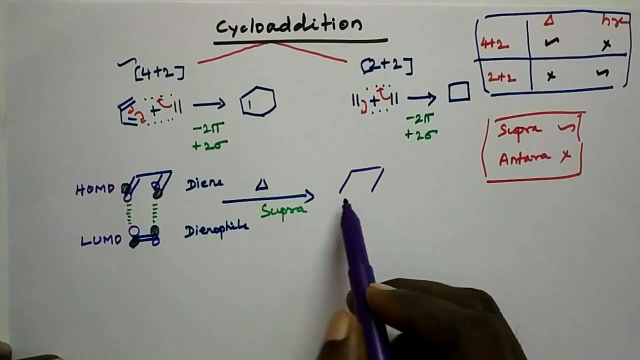 Supra. Supra is allowed, Antrafacial is forbidden. okay, Antrafacial is forbidden. So in this case we get supra when we perform the reaction thermally, So we get, so reaction is allowed. So we get the product. okay, We get the product, But the same reaction. 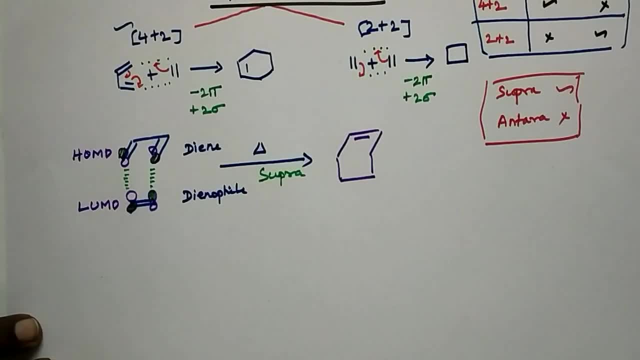 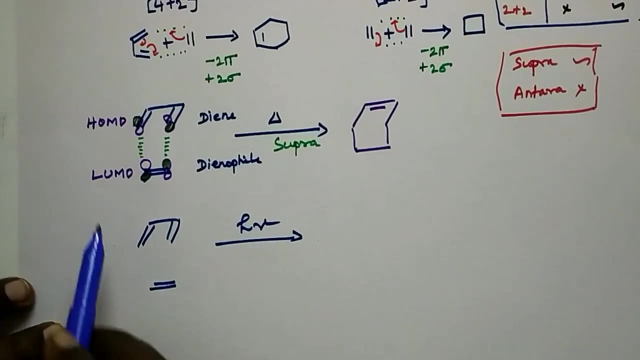 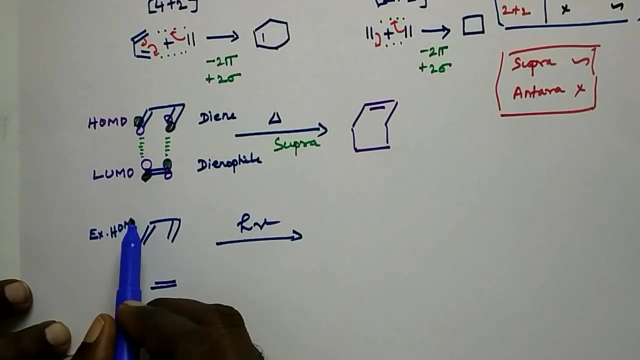 if we perform photo chemically, If we perform the same reaction, photo chemically, Photo chemically. Photo chemically means, you remember, instead of HOMO, we need to take what Excited HOMO? Excited HOMO. At the very first video, I think we have discussed about HOMO. 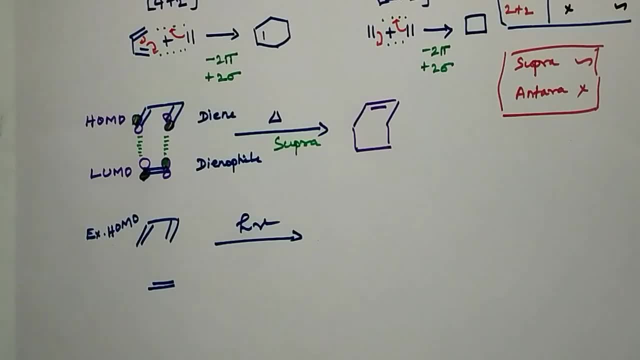 and excited HOMO. okay, When we go for photo, chemical condition electron from HOMO is visited to the next one, so and the next one becomes HOMO, so we call it has exited HOMO. okay, excited HOMO. and this one, as usual, LUMO. 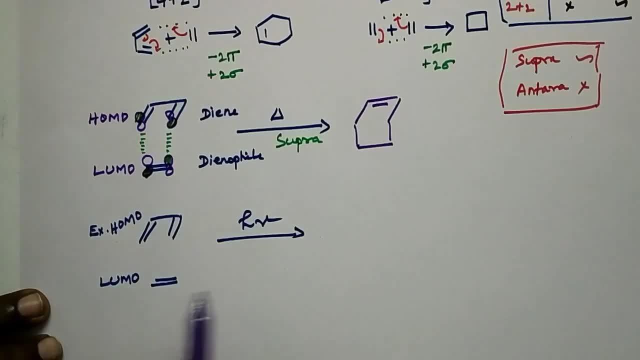 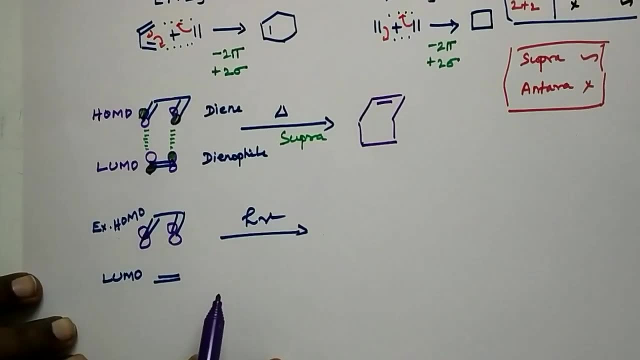 now how to draw the excited HOMO. Excited HOMO is nothing but LUMO, As i said. okay, so excited HOMO is nothing but LUMO And the LUMO you can draw as it is already drawn. 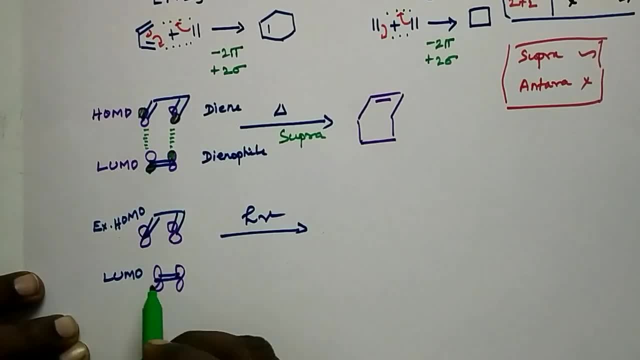 drawn here. you have drawn the Lumo, same way you draw it: Lumos and symmetry, but this excited homo. I mean Lumo. how can I, how can we draw? see homo is asymmetric, Apollo more should be. then Lumo should be symmetric, obviously because Lumos excited home. now see the orbitals. there is symmetry matches, but there is 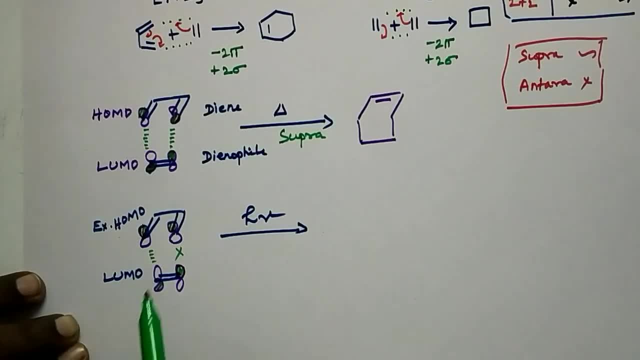 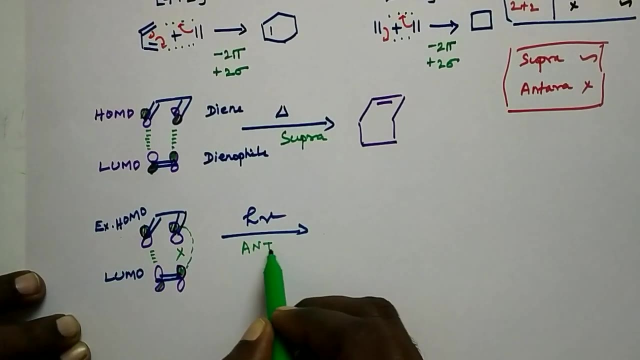 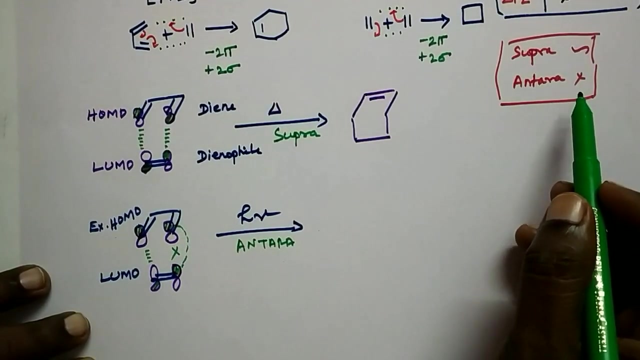 symmetry forbidden. supra, supra, supra facial. overlap is not possible here. if we want to allow the, if we want to achieve the overlap, okay, this has to come like that. okay, so it has to twist. that means antero facial, antero facial. as I told you, antero facial is not allowed for 4n plus 2 and 2 plus 2 antero facial. 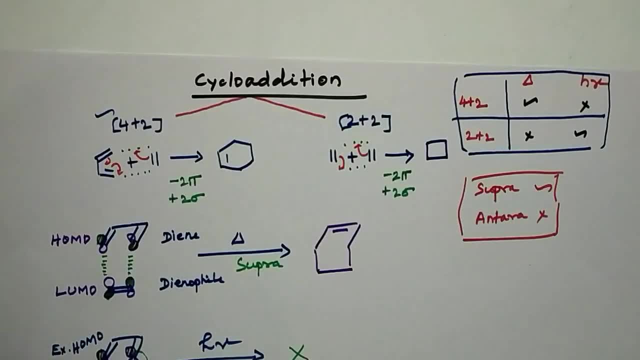 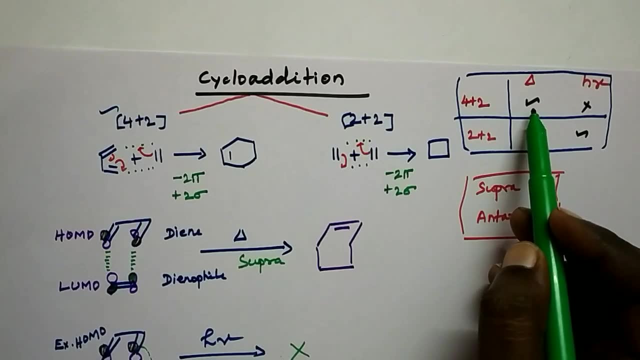 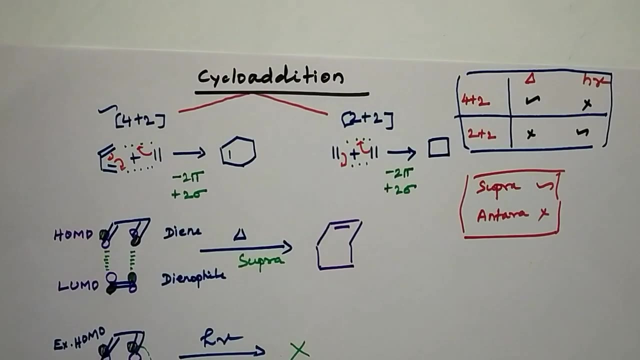 not allowed, so no reaction. that is why I have said four plus two: thermally allowed, photochemically forbidden, because thermally supra facial photo. chemically antero facial, okay, antero facial. and I want to remind you one more formula, the whole formula, what we studied at ca, at ca OCA. remember a ca oCA? 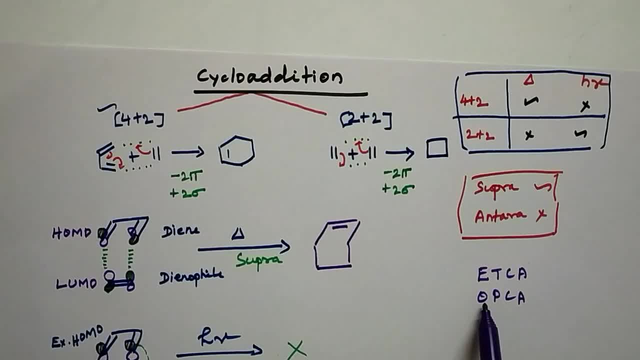 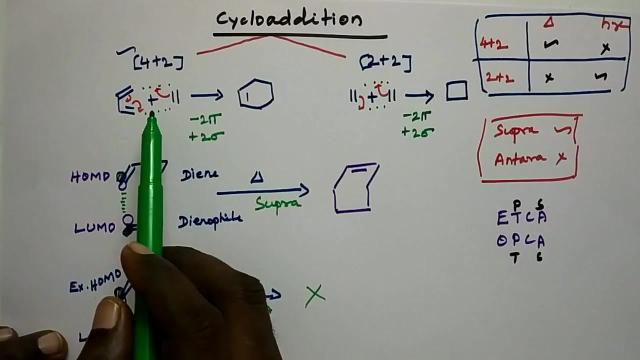 even thermal con rotation: antero facial hard photo con antero-facial Thermal. antero means photo-supra-facial, Photo-antero means thermal-supra-facial. Now look at this: 4 plus 2 cycloaddition, Overall how many pi bonds? 3 pi bonds Odd. 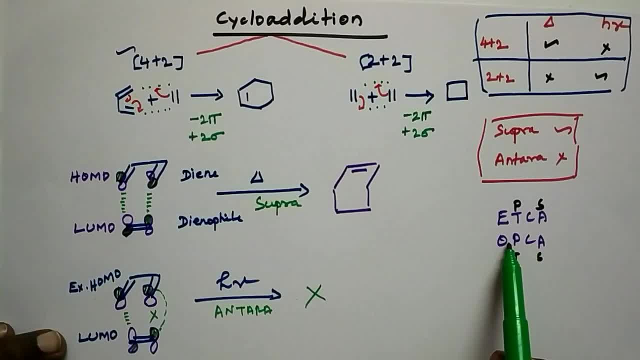 number: Odd photochemical, antero-facial, Odd thermal supra-facial. In our case antero-facial is forbidden, supra-facial is allowed. So odd thermal supra-facial is allowed. Supra-facial is possible only at thermal condition And that is why thermally allowed, photo-chemically. 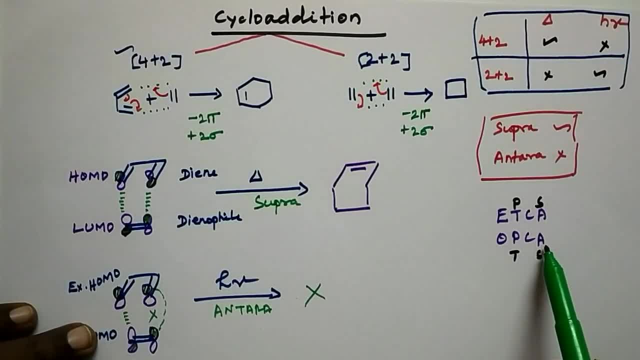 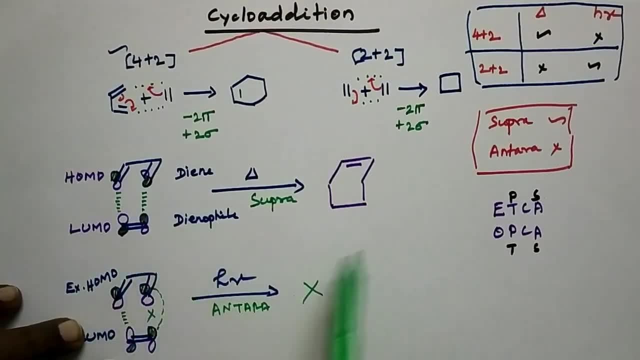 forbidden Because photo-chemically it is antero-facial, Thermally it is supra-facial. So, without drawing all these things, without these tables, simply yetka-otka itself, we can say whether it is antero-facial or supra-facial. If it is antero, you can say reaction. 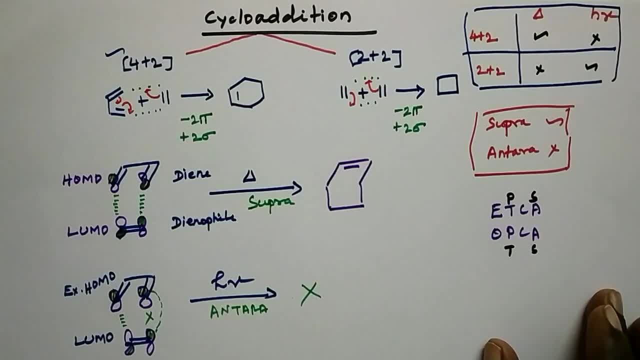 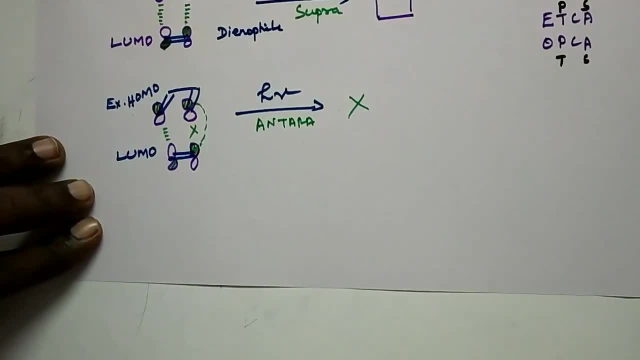 is forbidden. If it is supra-facial, you can say: reaction is allowed. Let us see the next one: 2 plus 2 cycloaddition. 2 plus 2 cycloaddition. 2 plus 2 cycloaddition. 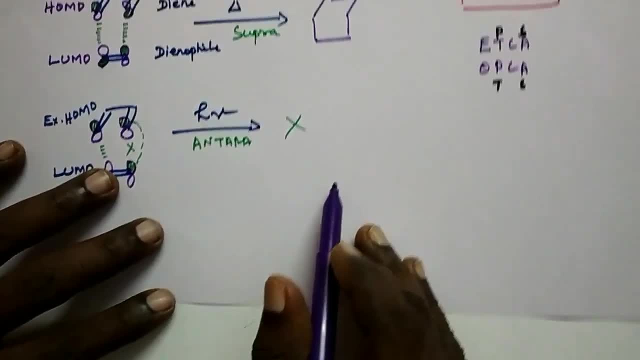 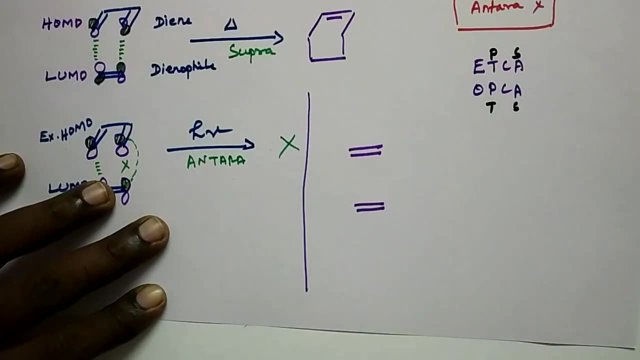 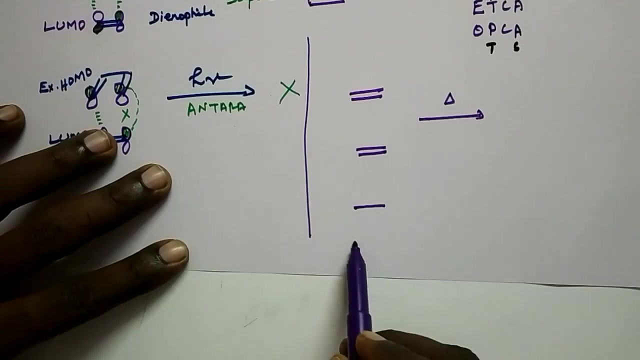 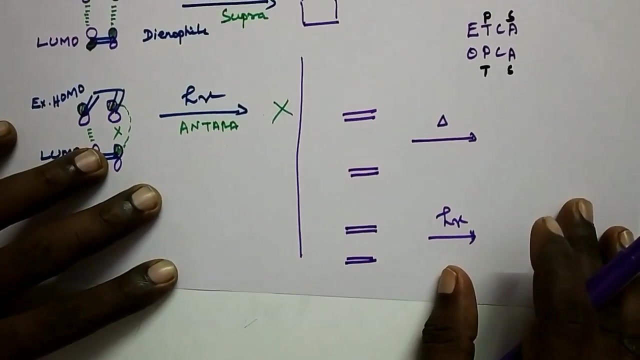 means- let me write it here- 2 plus 2 cycloaddition, 2 plus 2 cycloaddition Thermally and 2 plus 2 cycloaddition Photo-chemically. Photo-chemically, By yetka-otka itself. we can say 2 plus 2. 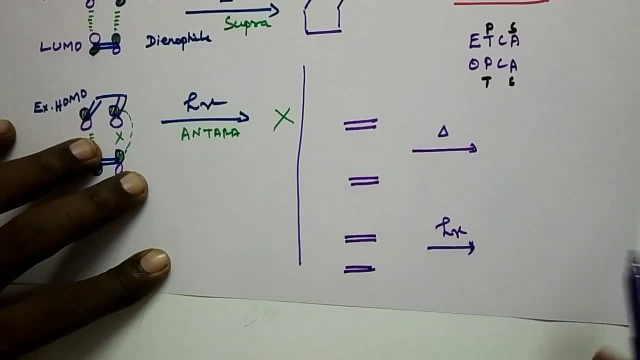 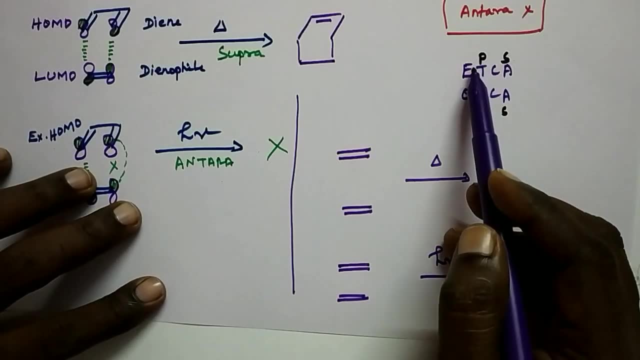 means how many 1, 2, 2 pi bonds. 2 is an even number, E1, E1, where do we get supra E1, photo-chemical supra? That means, this reaction is allowed only photo-chemically. 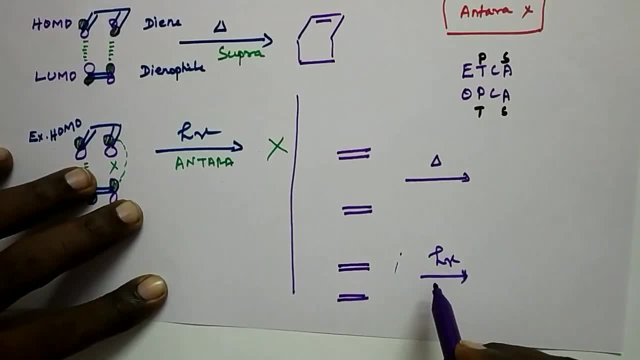 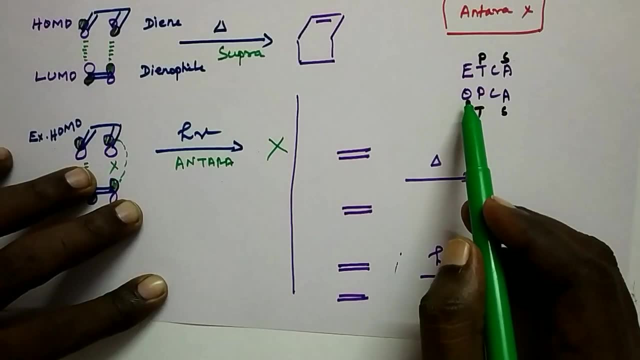 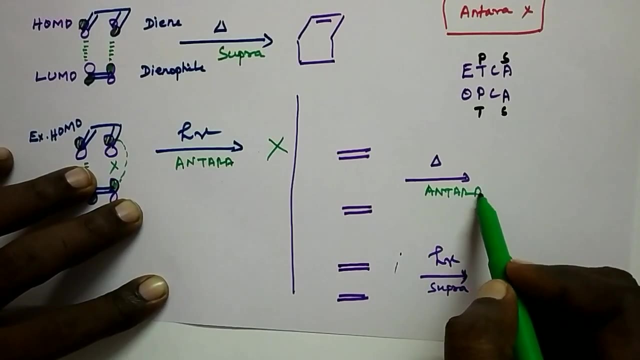 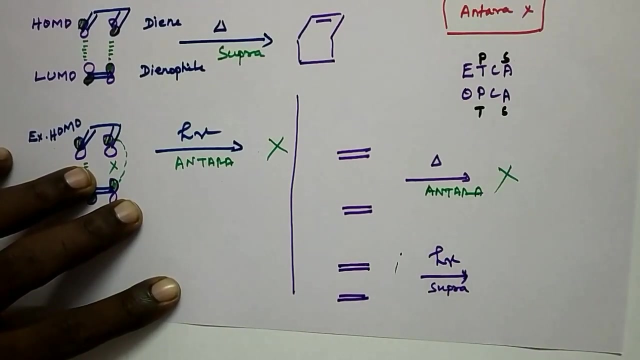 because supra-facial photo-chemical, here photo-chemical, we get supra, Photo-chemical supra And thermally E1, thermal antero, Here antero, That means supra-facial is allowed. So here you get the product Antero, no product. Supra-facially, you get the product Hope. 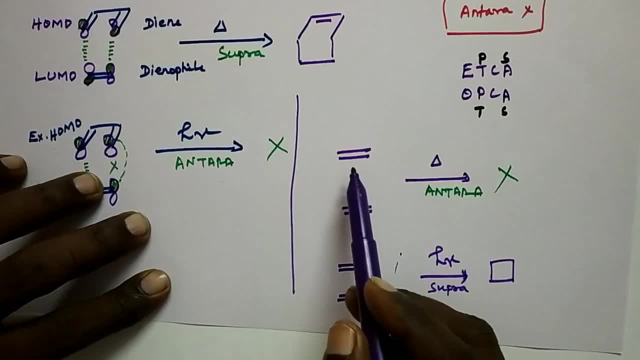 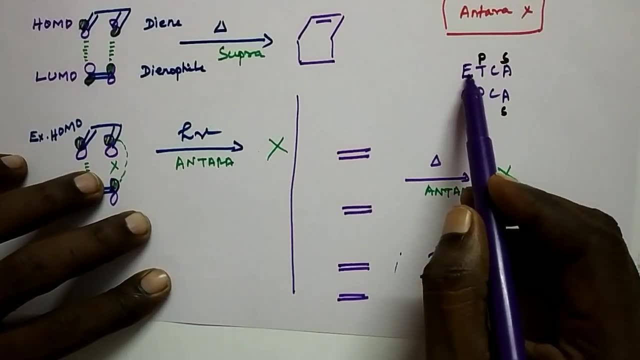 you understand Yetka-otka, formula: 2 plus 2 cycloaddition 2, 1, 2, 2 pi bonds. That means E1, number, E1.. E1, thermal antero, E1, photo-supra. In our case, supra is allowed, antero is not. 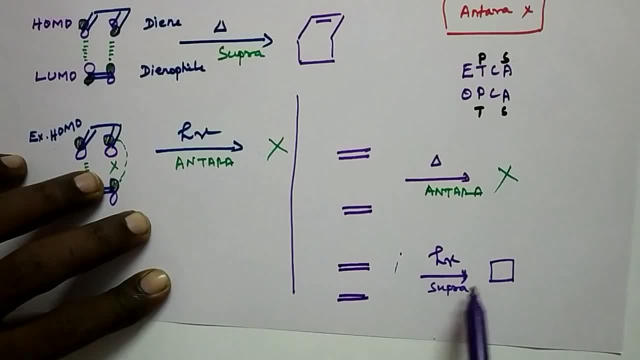 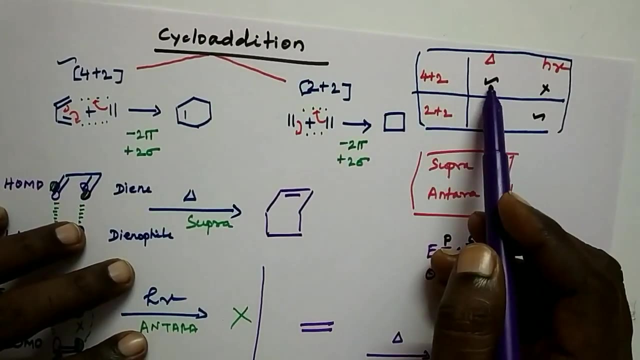 allowed Here. supra means photo, Photo-chemically supra we get product E1, thermally antero, Antero-facial is not allowed, So thermally this reaction is not allowed, no product. That is why I say 4 plus 2, thermally allowed, photo-chemically forbidden, But 2 plus 2. 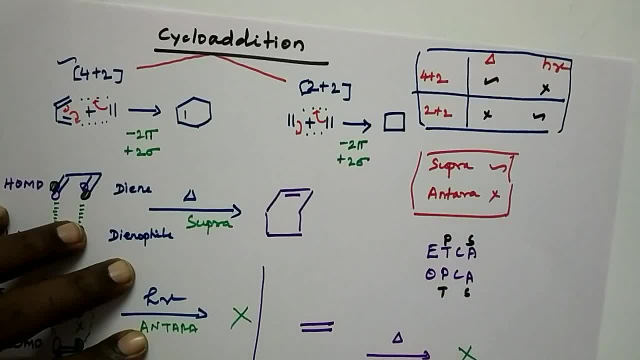 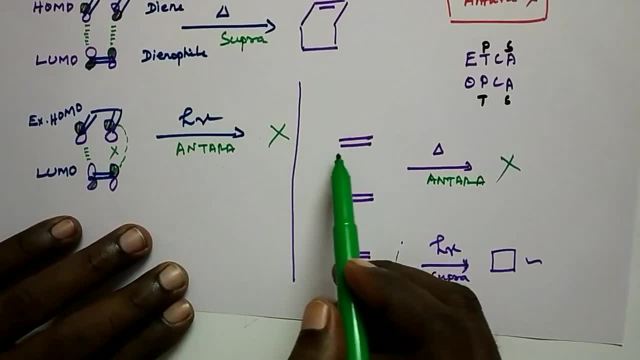 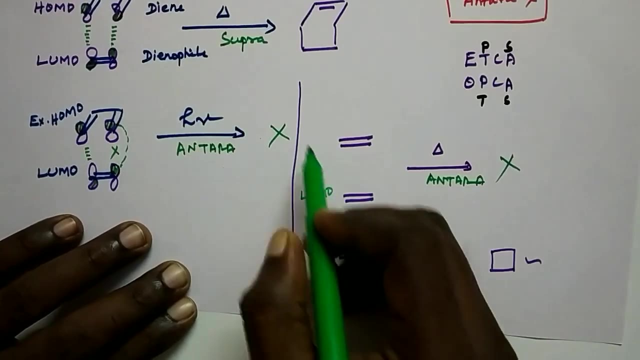 reaction: thermally forbidden. photo-chemically allowed. Photo-chemically allowed. For further explanation, just remember. just for clarification, for thermal means you should write, you should use what HOMO and LUMO, isn't it LUMO? and? 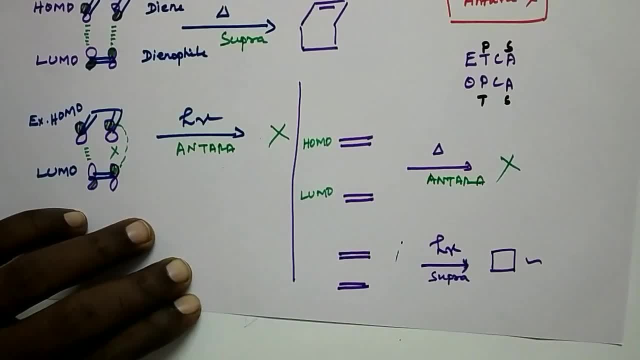 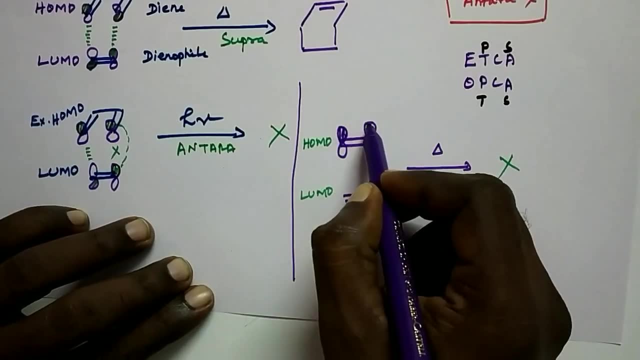 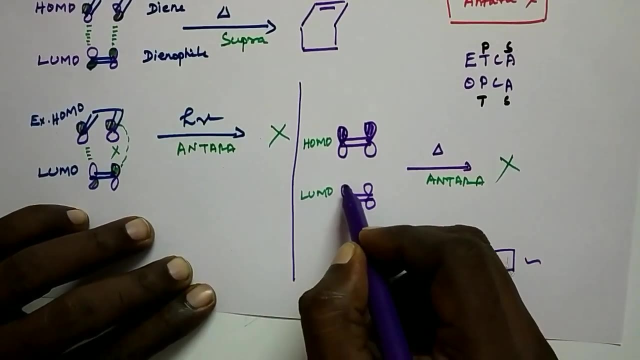 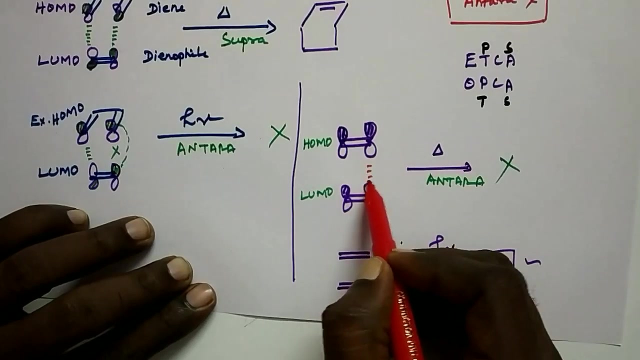 HOMO, HOMO, How will the HOMO be? HOMO is symmetric always for odd number of pi bonds. HOMO is symmetric means LUMO, LUMO and symmetric obviously. Now we see here symmetry allowed, here symmetry forbidden. 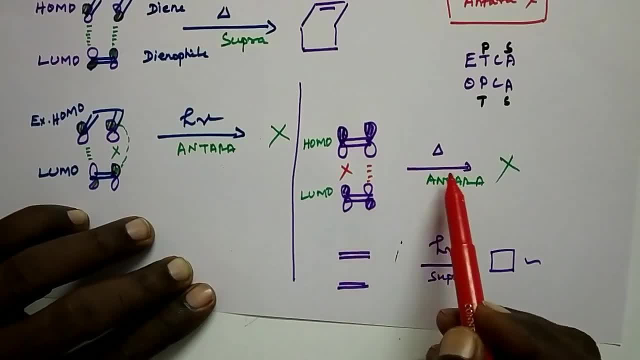 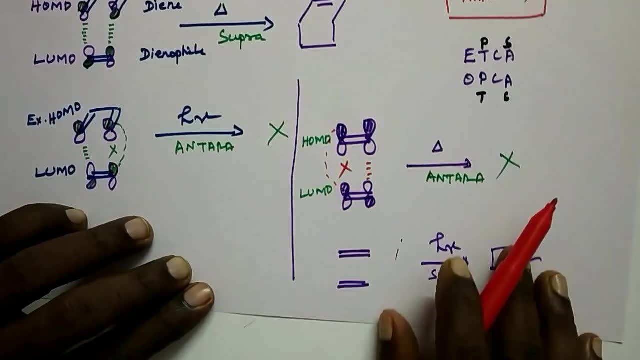 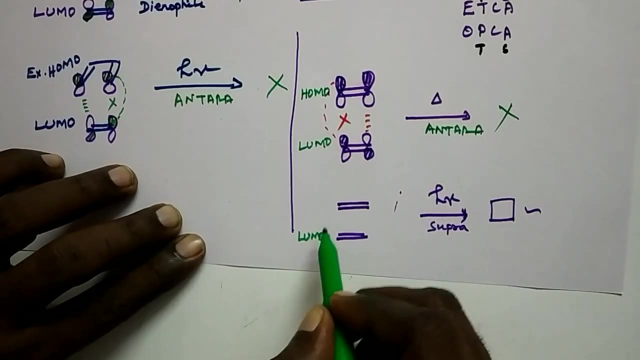 That is why thermal reaction 2 plus 2 thermal reaction not allowed because it is antero-facial. Okay, You have to overlap this way, But if you look at photo-chemical condition, photo-chemical means you should consider what LUMO and excited HOMO. 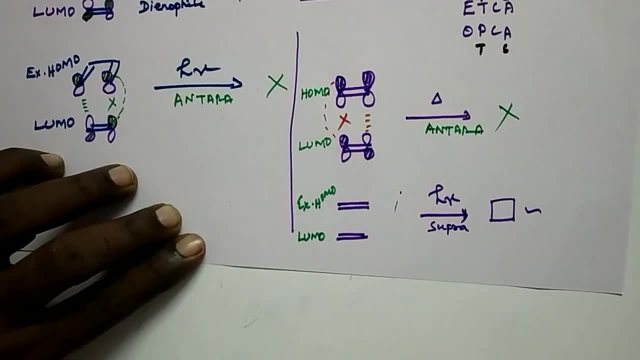 Isn't it? LUMO and excited HOMO LUMO, you know already, you have drawn the LUMO. LUMO is unsymmetric And excited HOMO means what Excited HOMO is nothing but LUMO. Okay So, 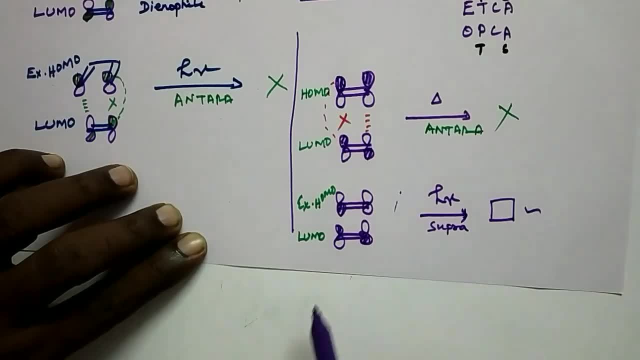 LUMO is unsymmetric. means here also LUMO unsymmetric. Okay, Now see the orbitals symmetry matches. Okay, You get the product. So here supra-facial, here antero-facial, So 2 plus 2 cycloaddition. 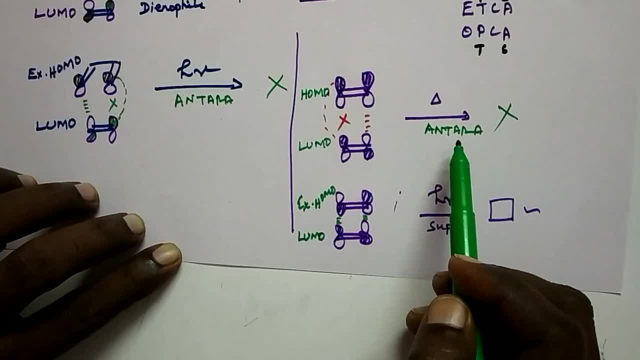 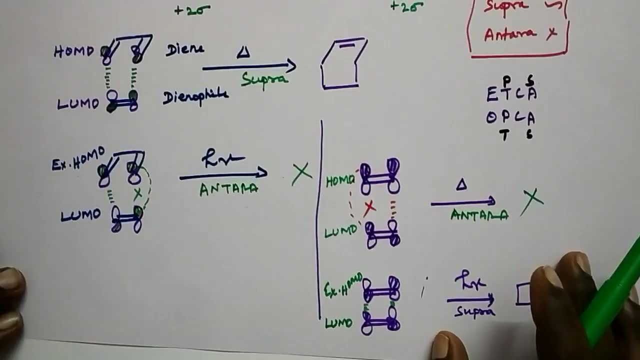 is thermally not allowed because it is antero-facial- 2 plus 2 cycloaddition- photo-chemically allowed because it is supra-facial. Why you get supra? why you get antero? Because you know by. 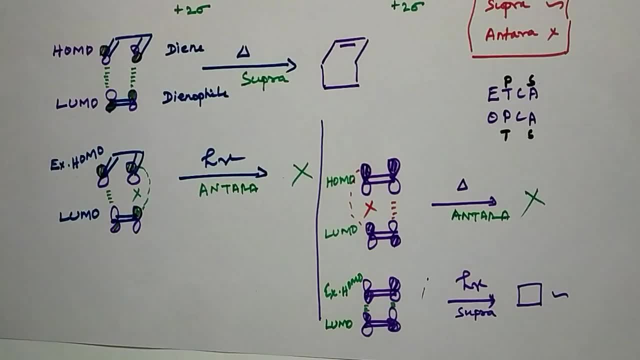 writing the orbitals: HOMO, LUMO orbitals. For thermal reaction, you need to take HOMO and LUMO. For photo-chemical reaction, you need to take LUMO and excited HOMO. Okay, If the symmetry matches, it is supra-facial. If it is not matching, it is antero-facial.